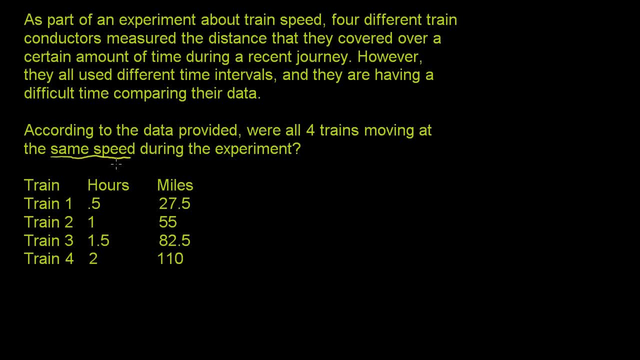 moving at the same speed during the experiment. So we just have to figure out what was the speed of all of these four trains, based on how far they went in this amount of time. And just to remind us, you might already know this, but 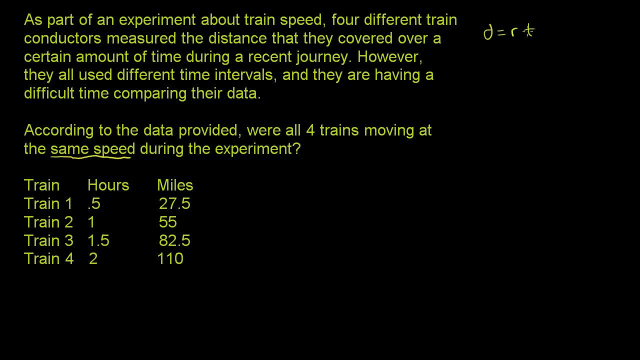 you know that distance is equal to rate times, time. Or if you were to divide both sides of this equation by time, I could do that. If you divide both sides by time, you could divide both sides by time. If you divide both sides by time, the times cancel out. 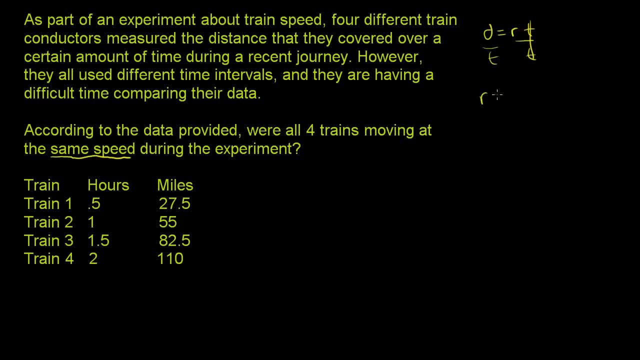 And you get: rate is equal to distance divided by time. Rate is equal to distance divided by time. Rate is the same thing as speed And it makes sense that it's distance divided by time. You've heard miles per hour or meter per second, or 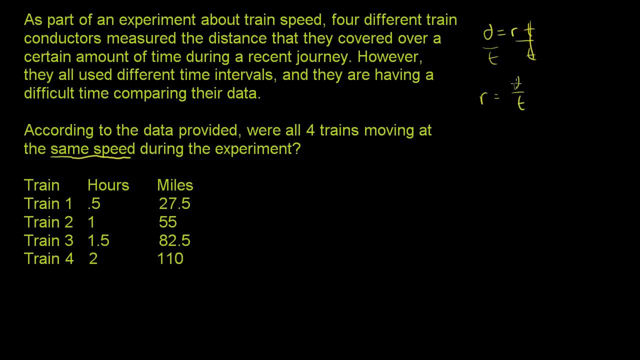 kilometers per hour. Rate speed is distance divided by time. So we need to figure out. so we can just use this: We can just divide the distance by the time For each of these trains and figure out what their speed was. 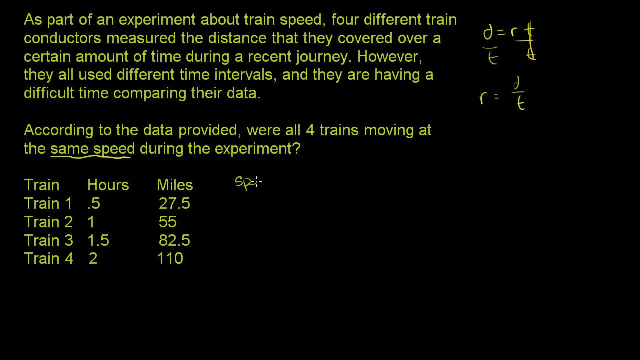 So let's do that. So let's write their speeds. I'll make another column for their speed right here. So what's this first guy? He went 27.5 miles in 0.5 hours. So once again, let's divide the distance for this train. 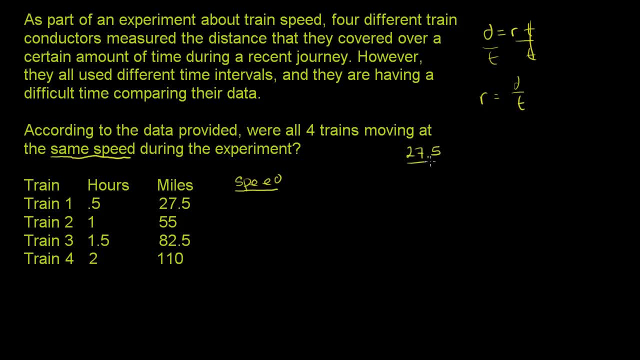 one. he went 27.5 miles in 0.5.. So if you divide something by 0.5, this is the same thing as 27.5 times 2.. Let me do it this way: Times 2.. 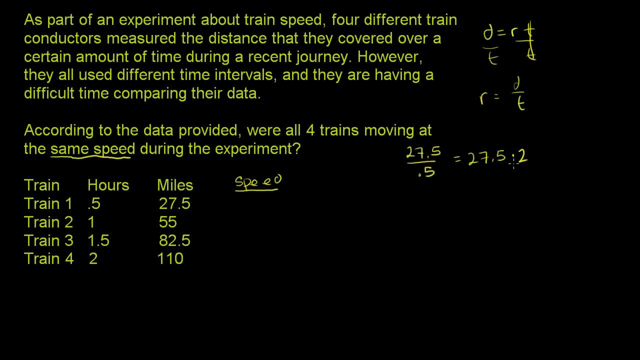 What's 27.5 times 2?? It is 55.. It is 55, and it is miles per hour, So his speed is 55 miles per hour. Now, this guy, this is pretty straightforward. He went 55 miles in exactly 1 hour. 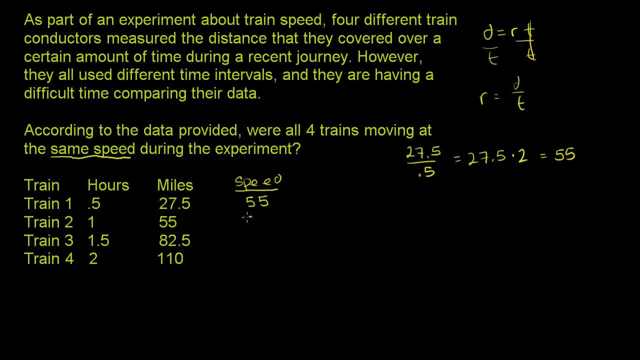 The distance divided by time is 55. So this guy is pretty straightforward. He's also 55. And you can put it in the formula: 55 is the distance. The time is 1 hour 55 over 1, 55 miles per hour. 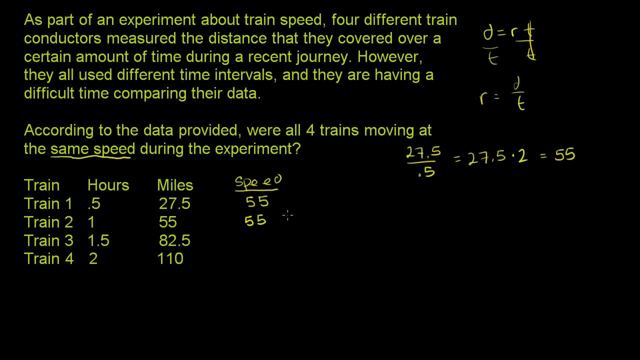 Now this guy went 82.5 miles in 1.5 hours. Let's see what that is. So he went 82.5 miles in 1.5 hours. So let's figure out what this is, And I'll have to do a little bit of decimal long division.